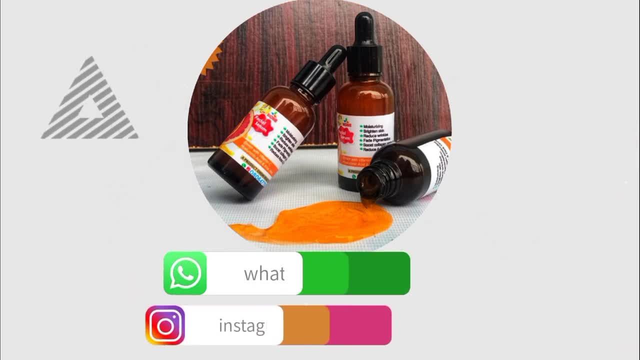 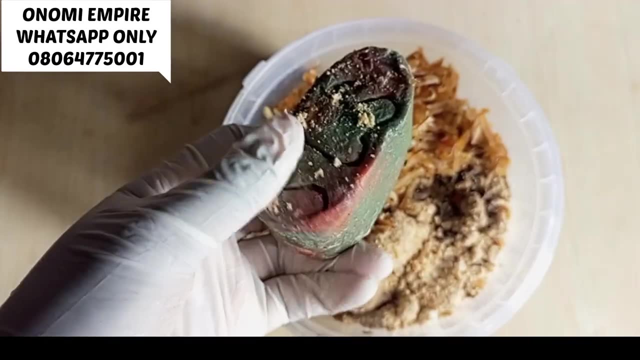 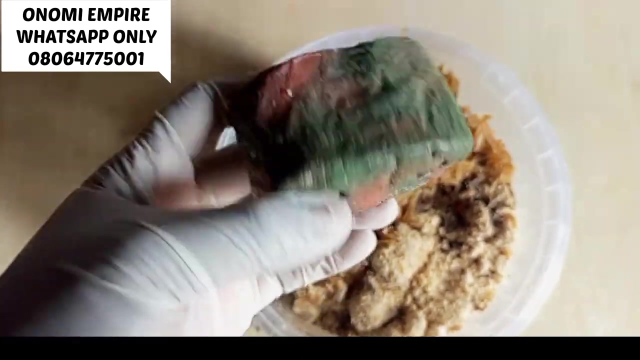 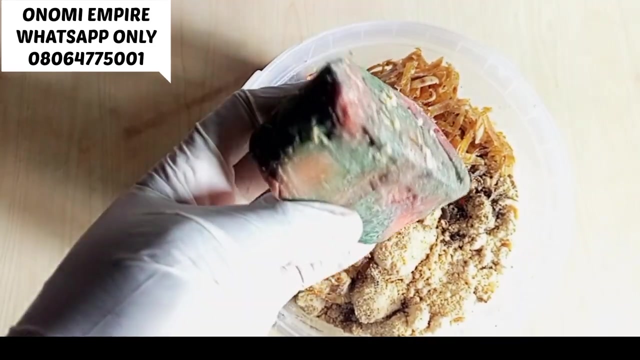 So, guys, these are my bases. This is my Kampala soap. This soap is an amazing soap. This soap will help fight rashes, ringworm, acne, eczema, body odor and any other skin issues- If your baby has anyone, and is so suitable for baby skin. So, guys, these are my bases. This is my Kampala soap. This soap is an amazing soap. This soap will help fight rashes, ringworm, acne, eczema, body odor and any other skin issues- If your baby has anyone, and is so suitable for baby skin. So, guys, these are my bases. This is my Kampala soap. This soap is an amazing soap. This soap will help fight rashes, ringworm, acne, eczema, body odor and any other skin issues- If your baby has anyone, and is so suitable for baby skin. 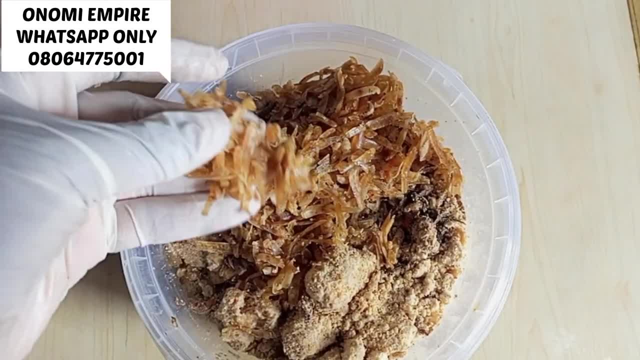 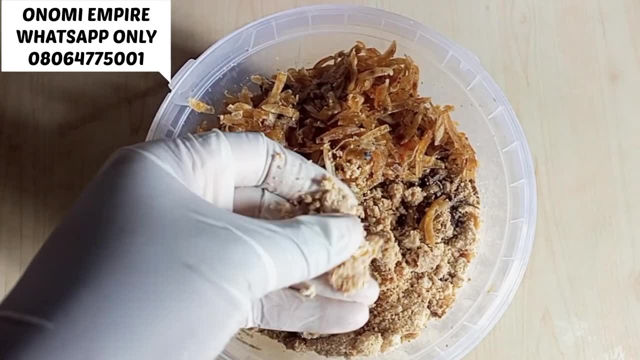 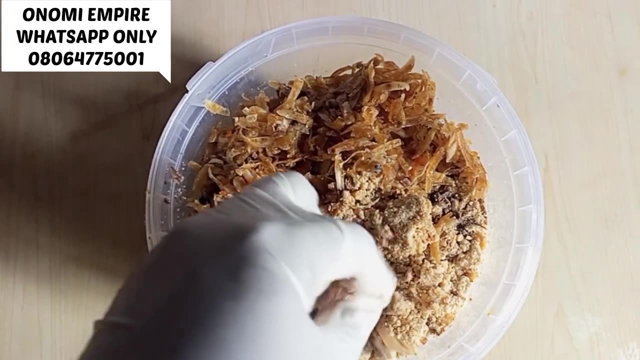 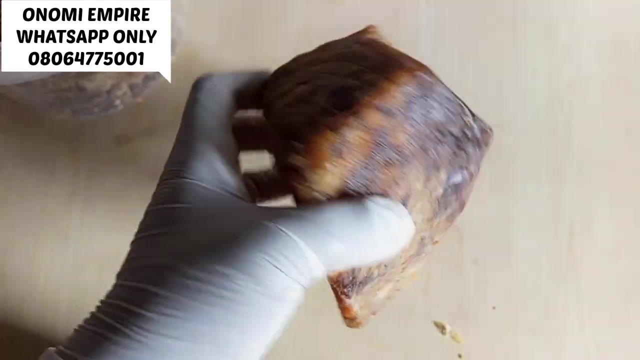 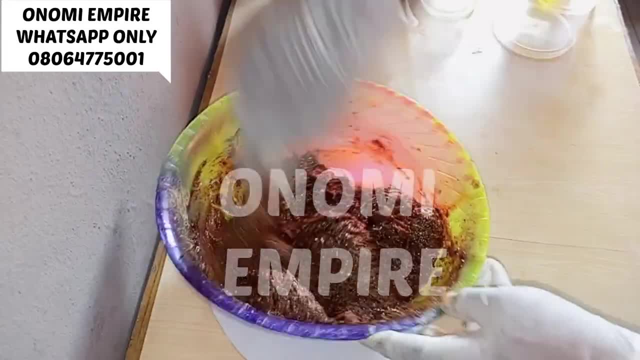 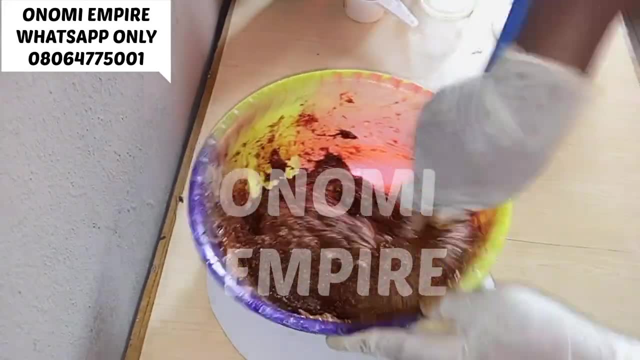 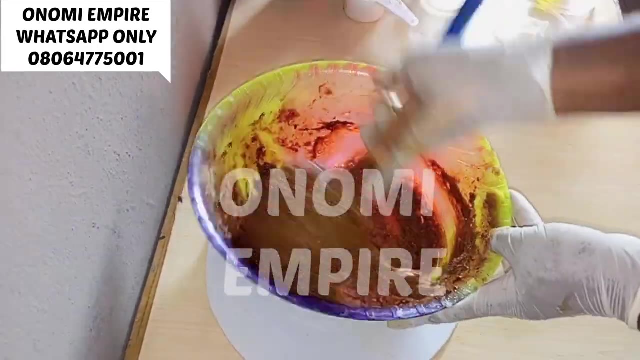 This is amazing. Now I'm mixing this up. This is exactly the consistency I want for this soup. I don't want it to be thick so that you can easily dip your hand into this soup and massage it on your baby's skin before you know, sponging their skin and washing it off. 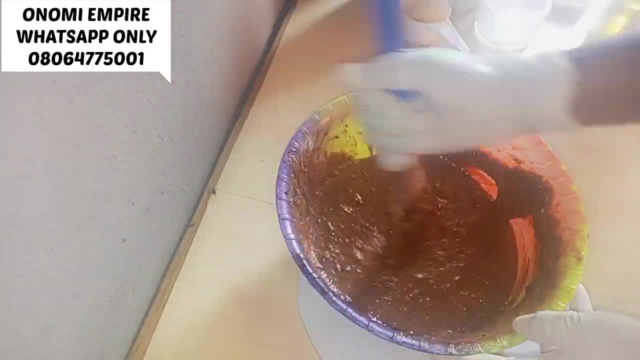 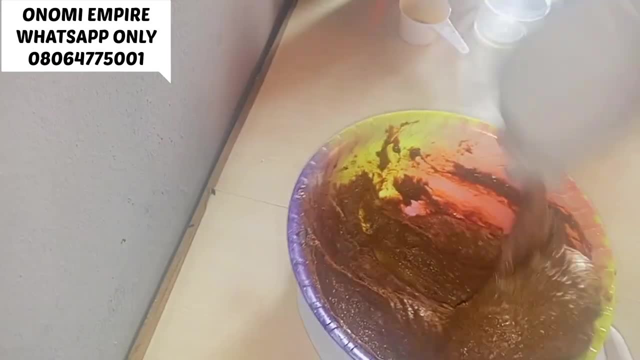 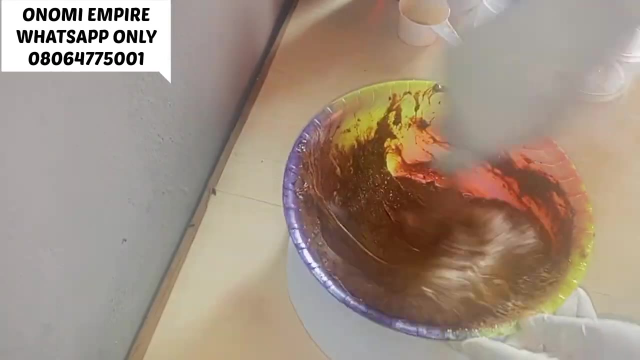 You can see very soft, But if you want yours to be- you know- a little bit harder than this, you could skip the powdered black soup and just use bar soup all through. So, guys, if you are yet to subscribe, Abba, please subscribe to this channel. 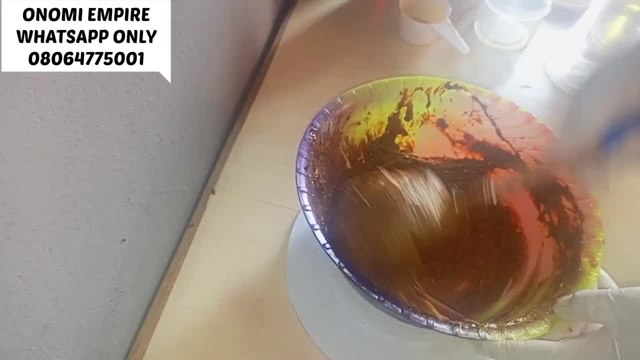 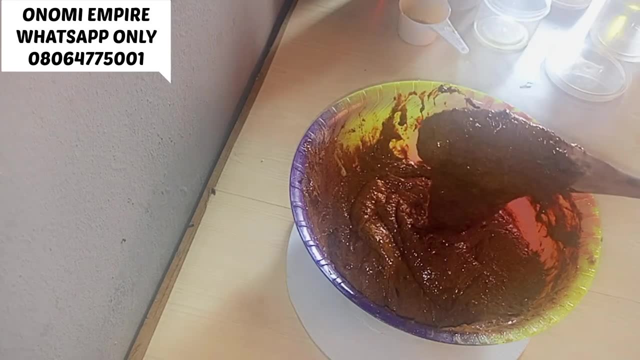 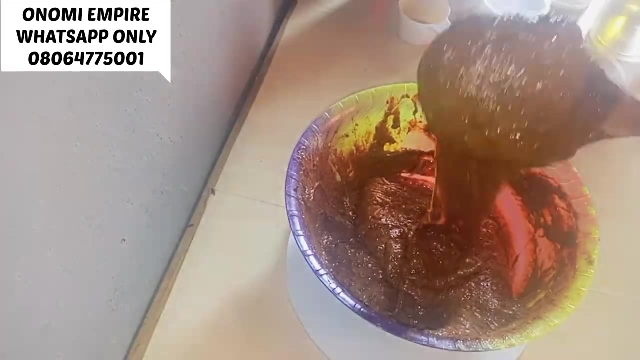 Like this video. Please hit the like button so that YouTube is going to push this video forward for me. Please, It's for free, Just help me hit the like button. Hit the like button Before we end this video right now. Like, subscribe and drop your comments in the comment section. 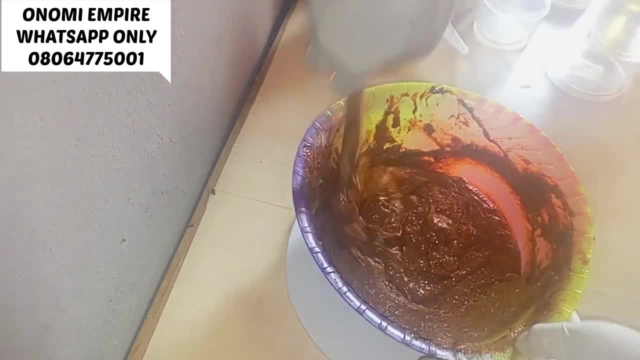 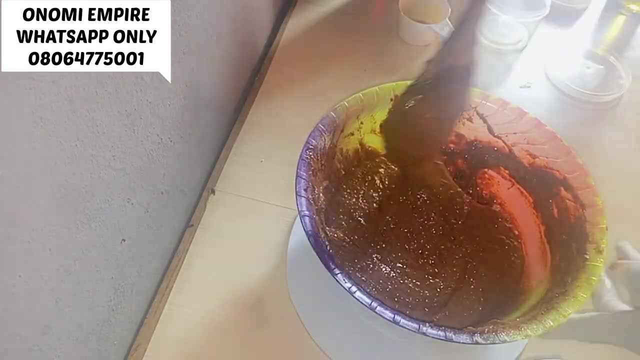 This soup is for one year and above. One year babies and above. If you want me to do a video on one year and below, please drop your comments in the comment section. I will do my very best to post that video. Now I'm dishing my soup into my container. 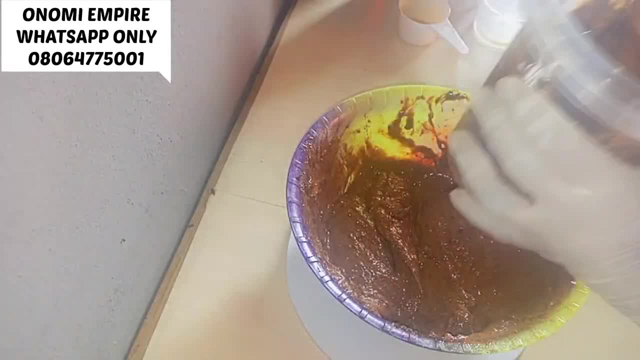 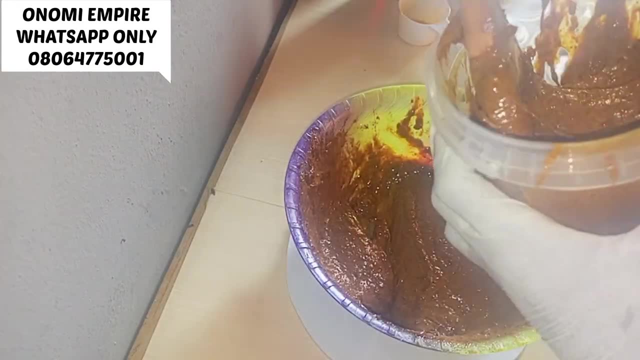 This soup. you can see how it is. It's not firm at all, It's very, very fluffy, And I love it. I didn't mix this with a hand mixer So that you will not say I don't have a mixer.